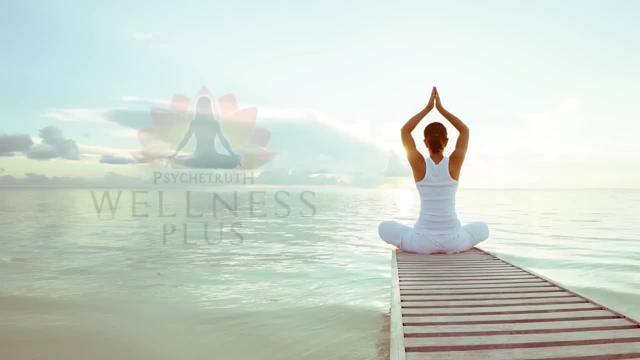 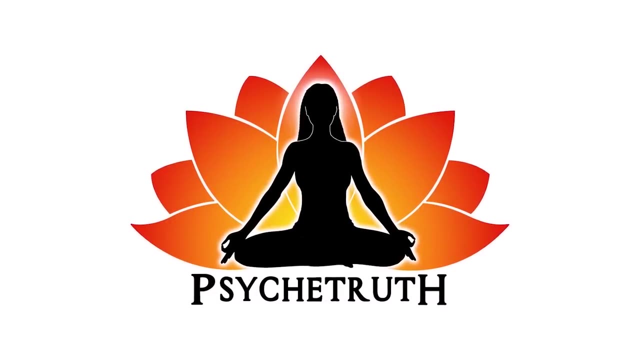 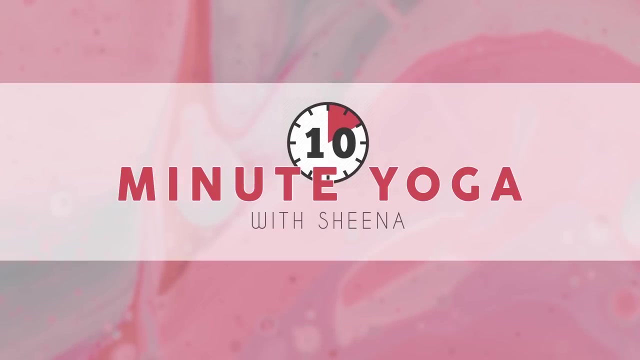 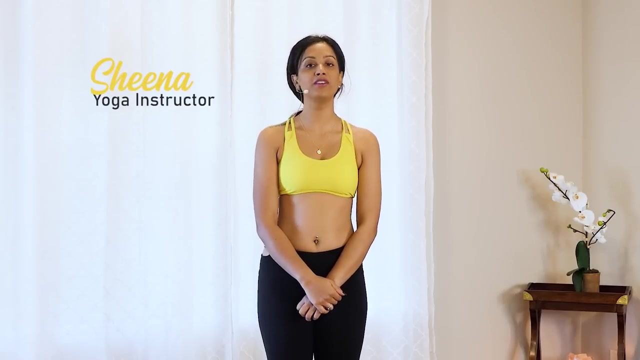 This video is made possible by our loyal Patreon supporters. Visit patreoncom. slash PsycheTruth. Hi guys, it's Sheena here, and today we're going to do a little 10-minute yoga series for weight loss. You can do this in the morning or in the evening, or both. It's pretty quick. 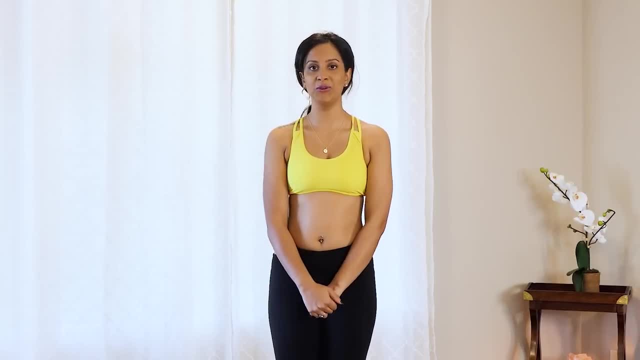 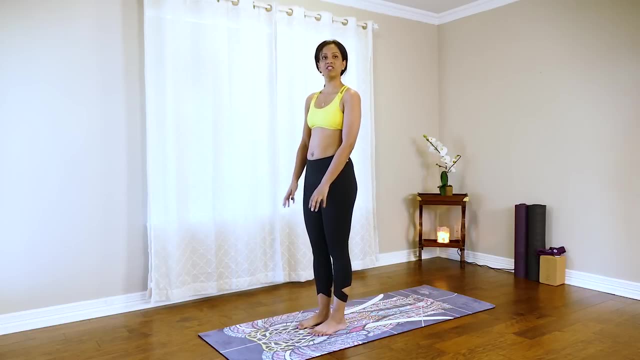 it's pretty low impact and it's a great little flow to incorporate into your day if you're looking to lose some weight. So let's go ahead and get started right away. We're going to go ahead and start standing at the top of our mat and let's inhale those arms nice and high. 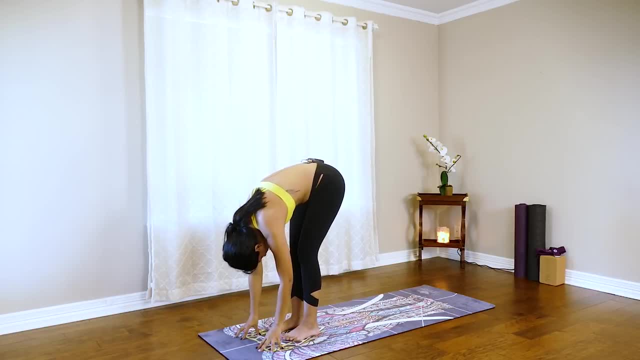 and we're going to exhale. hinge at the hips forward fold. We're going to inhale for halfway. lift Hands, come below the knees and exhale flat back forward. fold. We're just going to warm up and inhale slowly lower down onto the belly. hands stay beneath the shoulders. Inhale for. 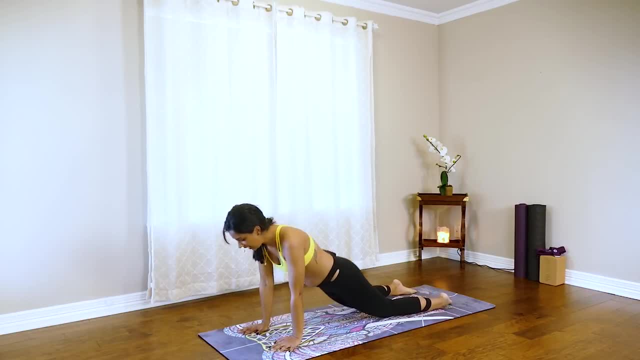 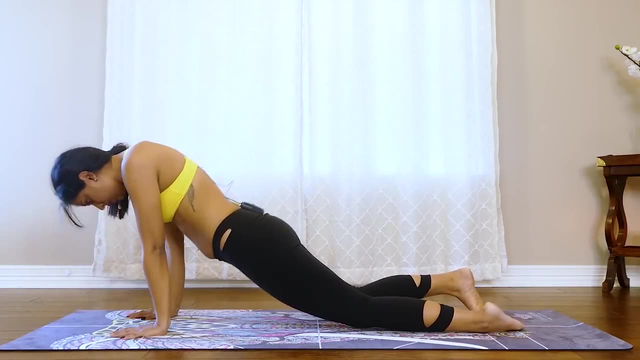 baby cobra chest comes to the sky and exhale, shift the hips back to the heels for a child's pose. We're going to do that a couple more times. Inhale slowly, roll to cobra. head comes last. 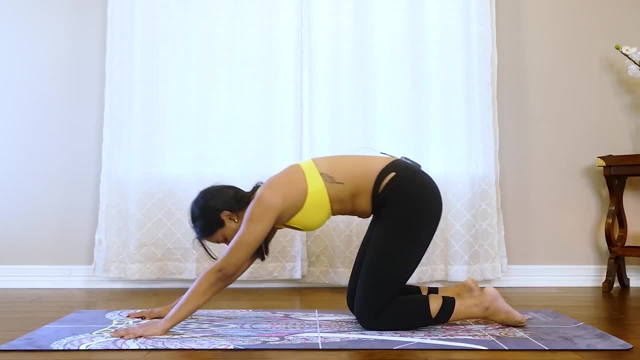 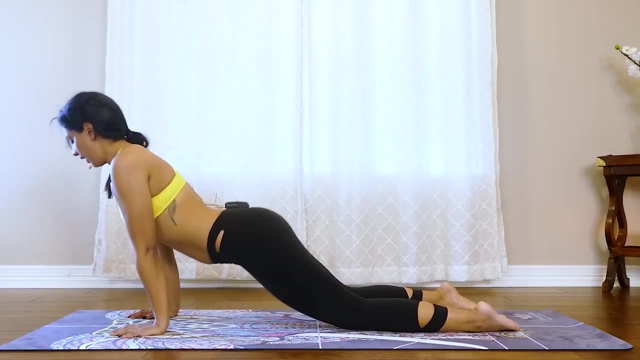 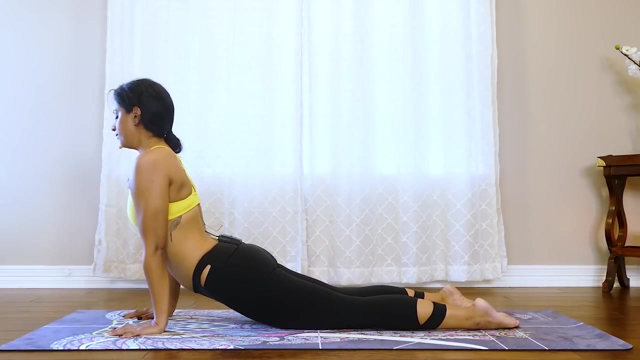 open up the shoulders and exhale. roll Back to child's. Just warming up the spine here. Inhale to cobra. Exhale child's. Begin to create a rhythm for your breath. Exhale child's Last one here, Inhale cobra. 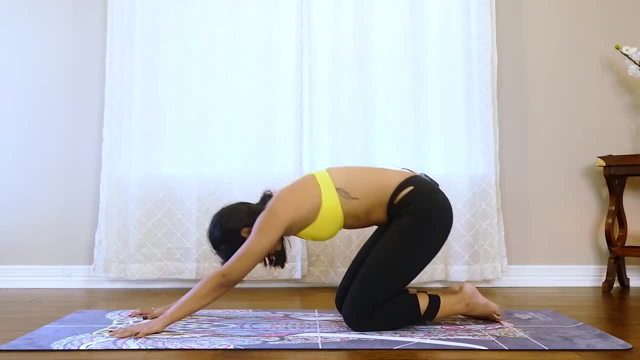 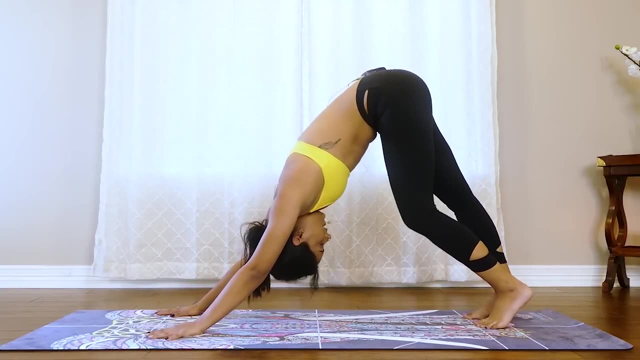 Exhale child's. This time on the inhale we're going to tuck the toes and shift the hips back to the sky Downward facing dog. Go ahead and pedal out the legs here From our inhale in down dog. 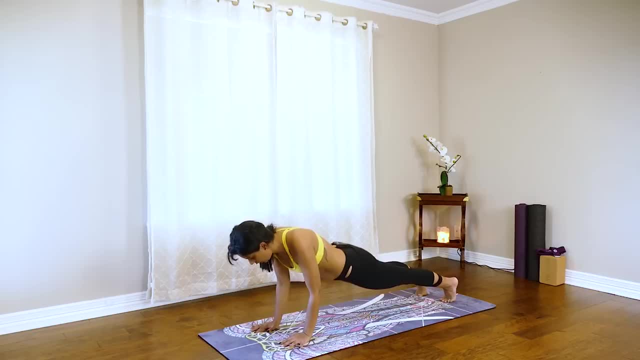 we're going to roll the length of our spine to a plank. come down to cobra, onto the belly, Inhale up, Exhale, tuck the toes down. dog, Let's do that a few more times, Slowly rolling. 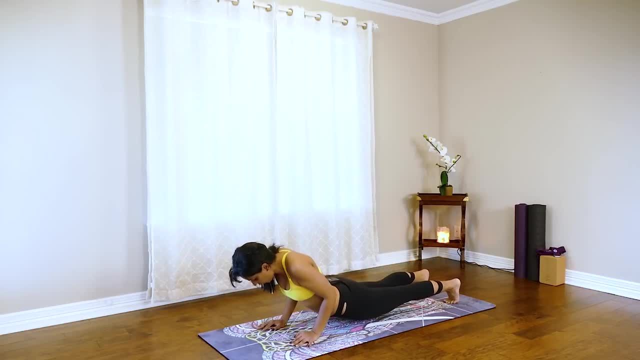 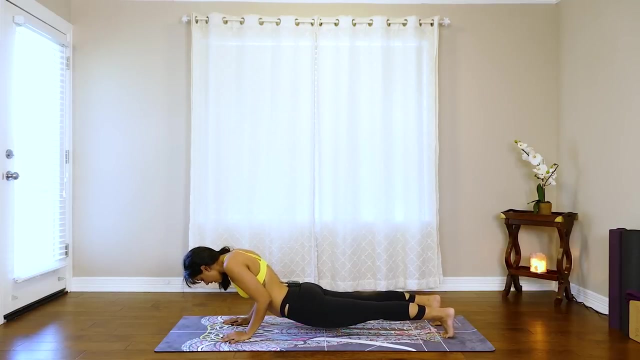 the length of the spine. head comes last lower down onto the belly. Exhale- boxes inhale for your baby. cobra Exhale- tuck the toes down. dog Inhale: come up onto the stippy toes, Just shifting the position of the hips- Exhale lower down. 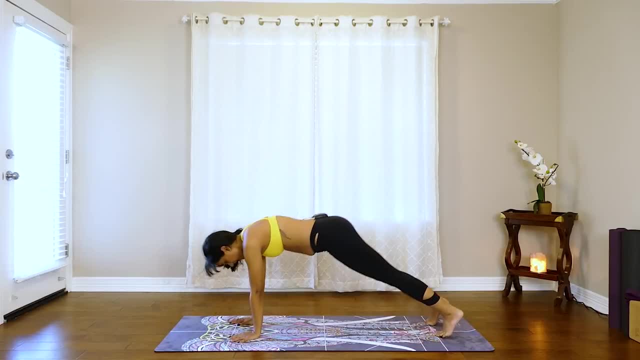 Inhale to cobra, Exhale down dog. Let's do that once more. Inhale roll, Exhale down. Inhale cobra. exhale down dog. one inhale and down dog. guys keep pushing that mat away. exhale and down dog, let's. 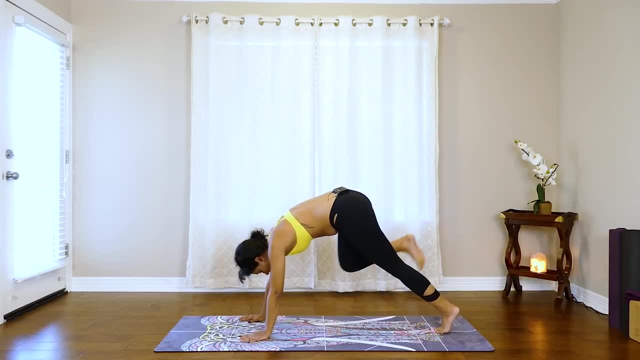 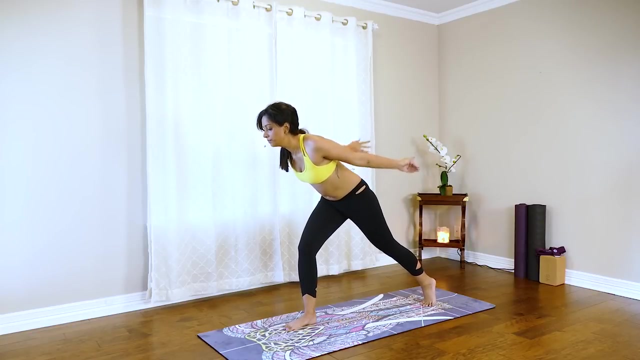 inhale. reach that right leg high and on the exhale we're gonna step it through the hands for a low lunge inhale. find your balance, rise to your high lunge and exhale. we're gonna swing those arms back, engage through the fingertips, airplane lunge, inhale those arms high, high lunge, exhale airplane. 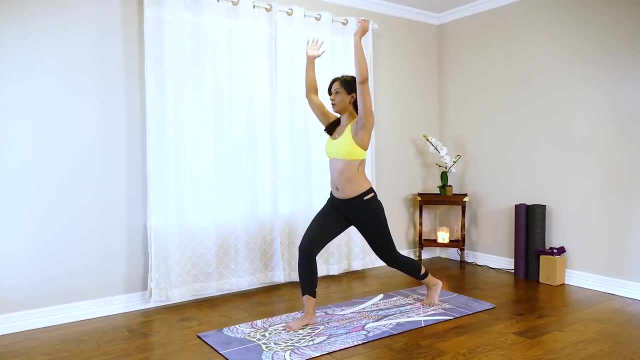 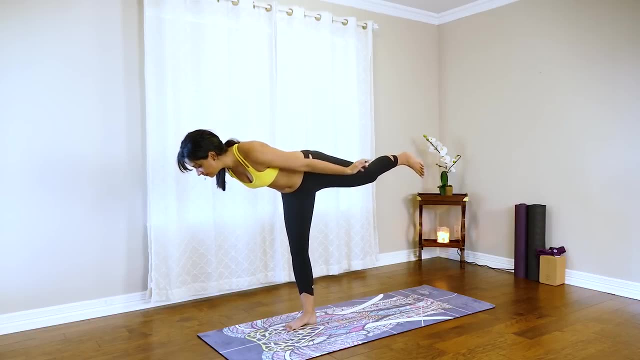 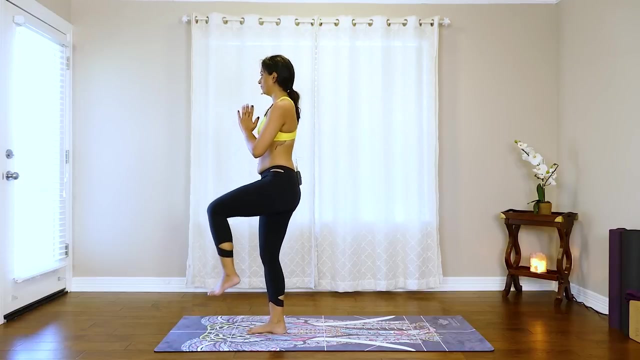 lunge one more. inhale arms high. this time we're gonna take a full airplane balance. get firm in that right leg. lift the chest one. inhale an airplane and exhale mindfully. swoop that left leg through, stork pose. let's do that twice more. inhale. 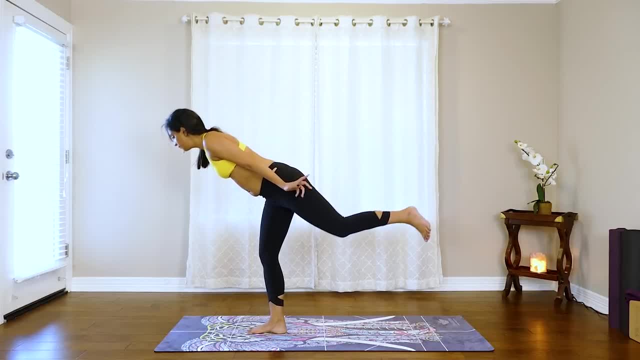 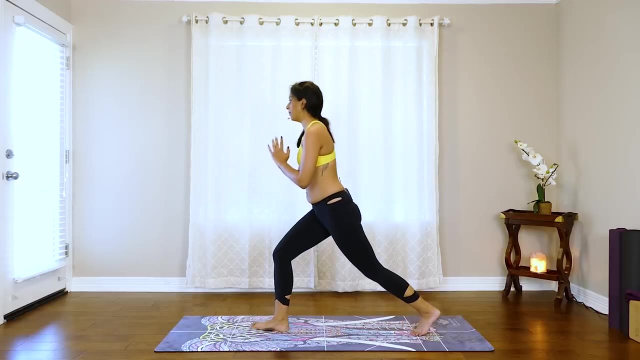 airplane. really drive through that left heel- exhale stork. it's okay if you wobble. last inhale airplane exhale stork, coming out the same way we came in. inhale. step back to your high lunge exhale frame the right foot with the hands. one breath, one movement. guys inhale, take a vinyasa. 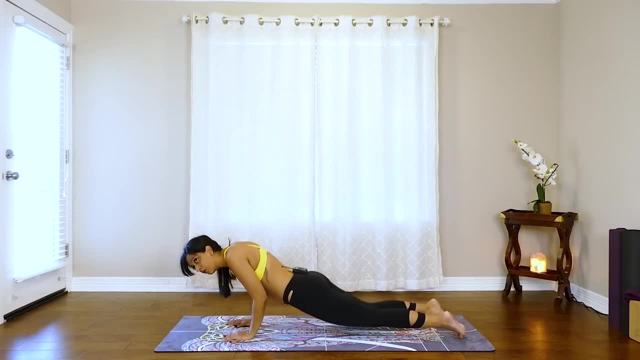 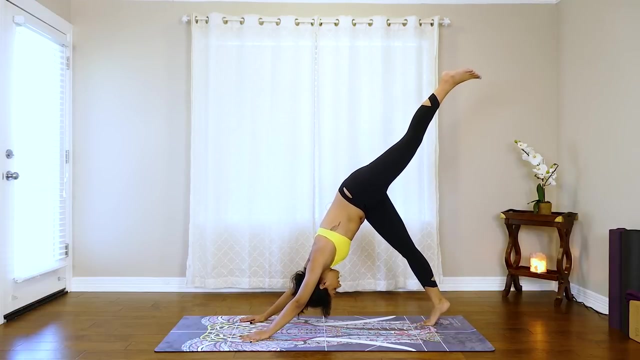 high plank exhale lower, halfway down or all the way down exhale. you can also keep the thighs on the mat for modification inhale for modified up dog or up dog exhale to down dog right to the other side. guys, let's inhale that left leg high and exhale step. 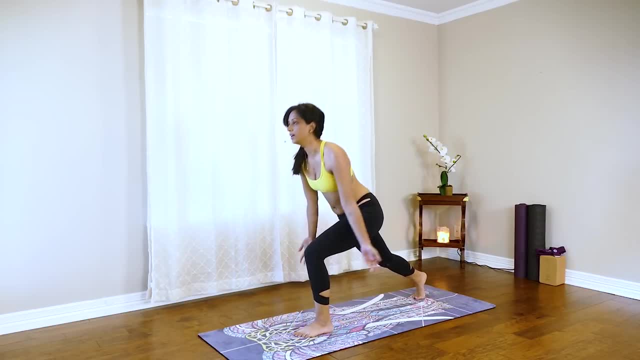 it through the hands. low lunge- inhale. find your balance. high lunge. keep those shoulders down, away from the ears and exhale. shoot those arms back. airplane lunge. we're kind of leaning over our left thigh here. inhale arms high, airplane, I'm sorry. high lunge, exhale. airplane lunge. last inhale high. 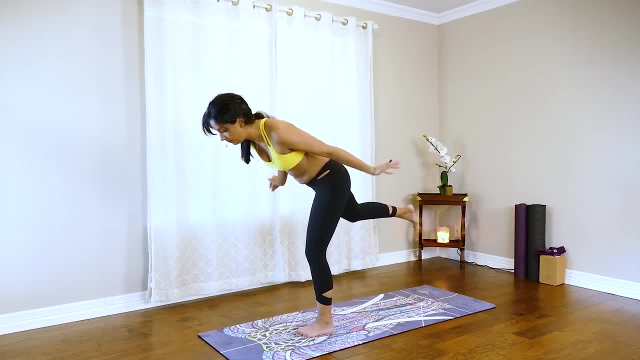 lunge and this time we balance: full airplane, one inhale an airplane. flex those right toes, exhale to stork. swoop that right knee up into the chest- inhale airplane, exhale, stork. last inhale airplane, exhale. step the right foot back high lunge, inhale: frame the left foot with. 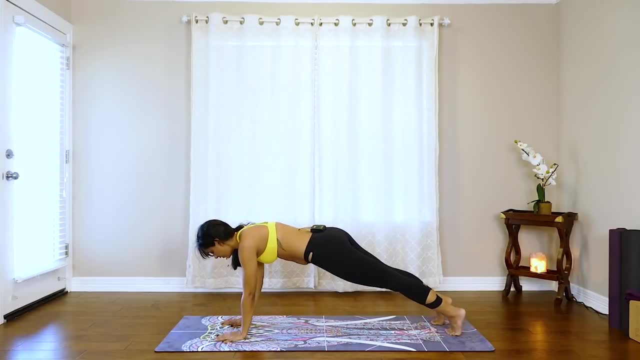 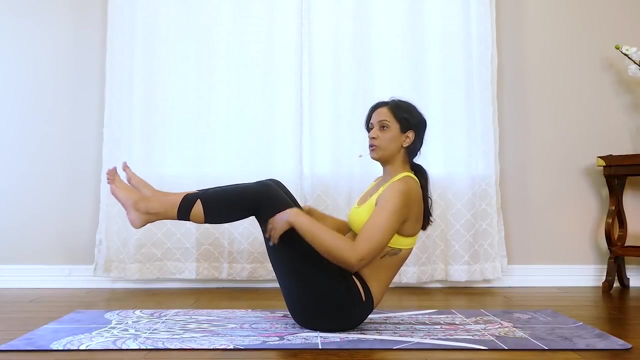 the hands, exhale. step back, high plank. take a vinyasa: inhale up dog, exhale down dog. one inhale and down dog guys. one exhale and down dog. look past your hands, bend your legs, see if you can jump to your feet and we're going to come to seated. we're going to come straight into our high boat. 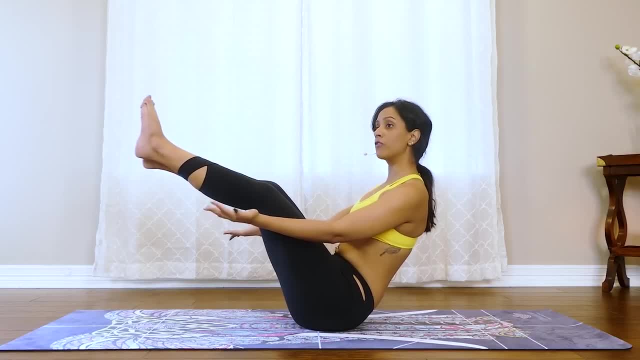 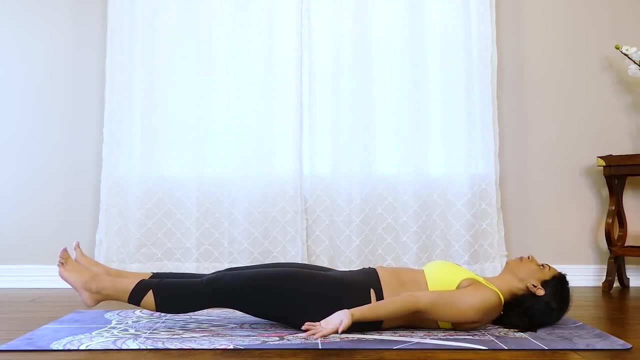 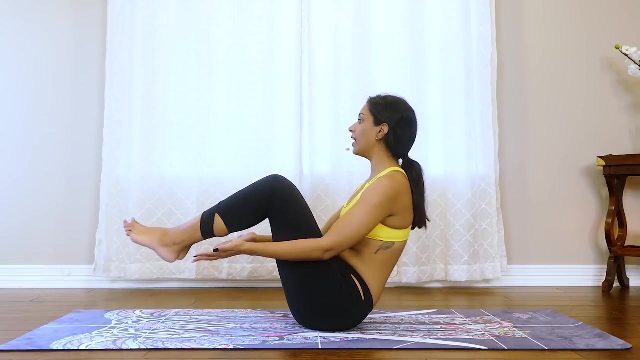 guys. so bring those legs to 90 degrees. you can also straighten them for the most advanced version. we inhale: sit up nice and tall in our high boat. exhale feet and shoulders. hover low boat. inhale to high boat. exhale low boat. keep that core engaged. inhale high boat. exhale low. two more: inhale high. 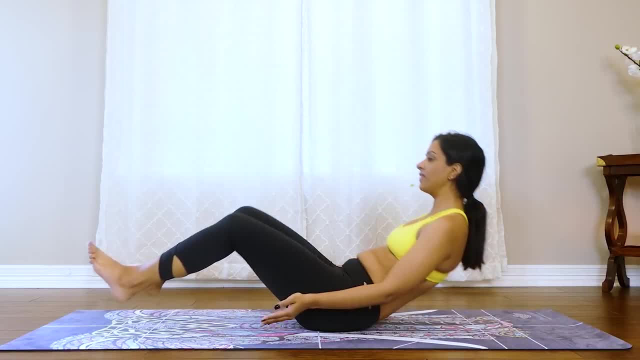 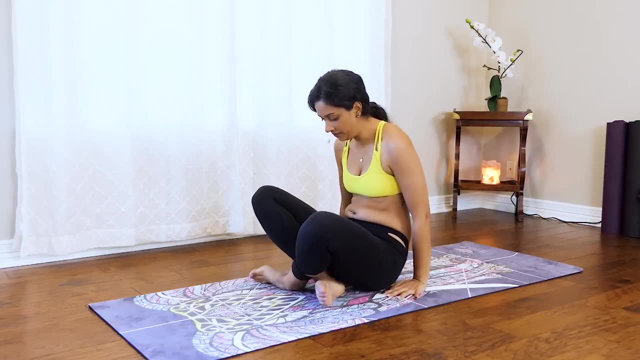 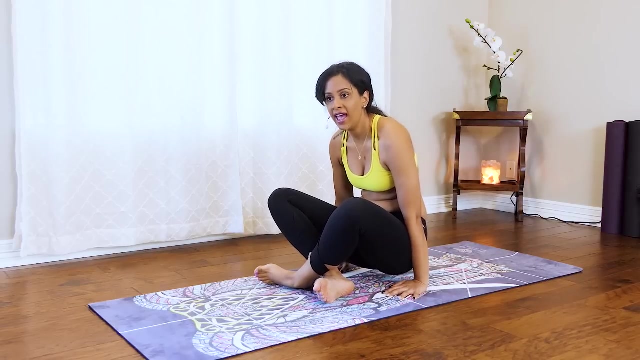 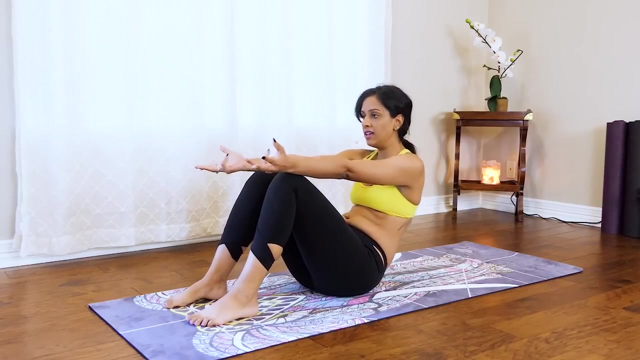 exhale low. last inhale high, exhale low. we're going to inhale high. cross the feet, bring them close into the body, and we're going to lift the hips off the floor for five, four, three, two and one. go ahead and come down from here. let's lower down onto our backs, guys. so plant the feet, slowly, roll down. 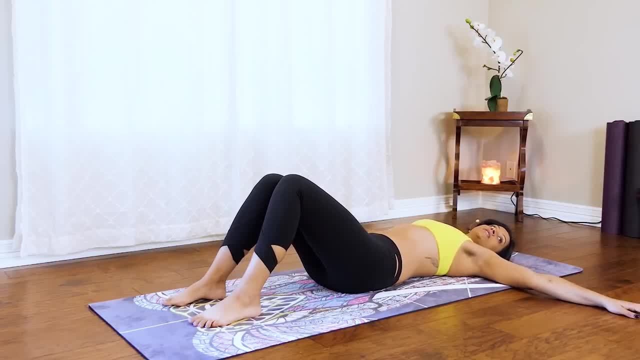 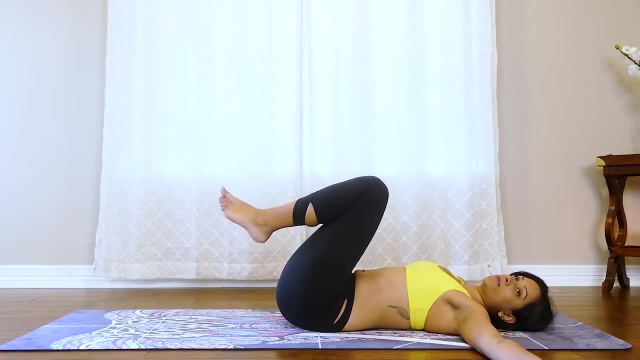 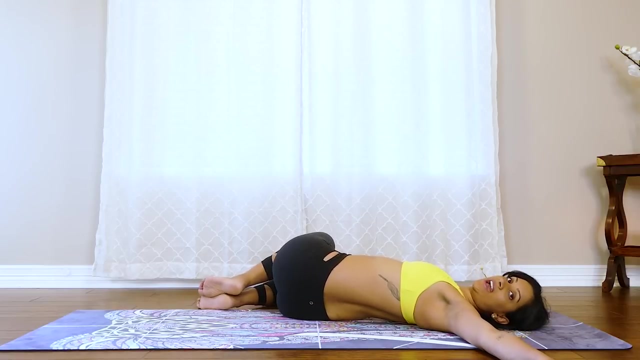 onto the back. we're going to bring the arms out to T and let's just cool down, taking a supine twist. so first let's bring the knees into the chest and then we're going to just roll them over to the right side. you can cactus the arms here. 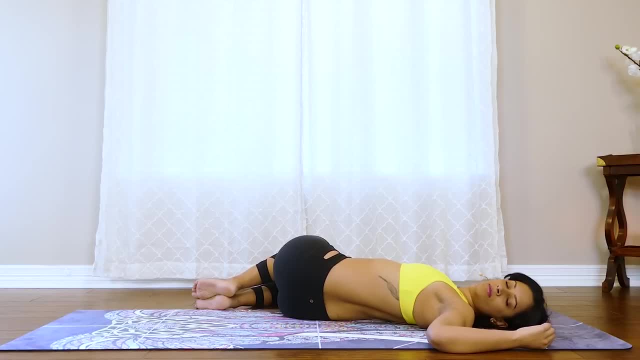 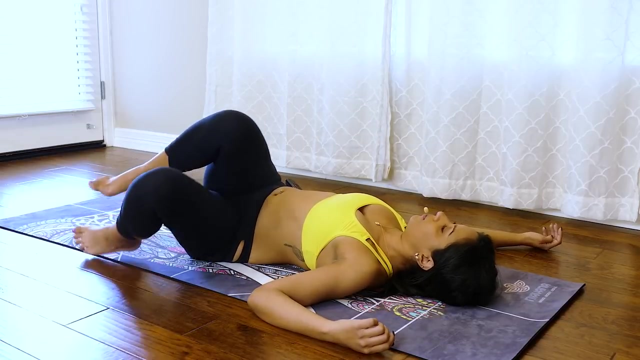 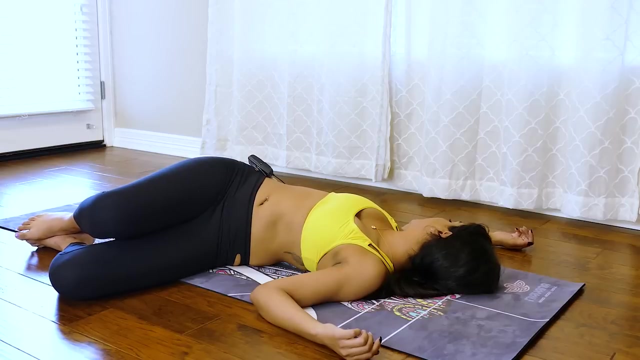 or straighten to T. two more breaths here, foreign. and on your next inhale go ahead and bring those knees into the chest and on the exhale lower them over to the left, looking over the right shoulder. inhale here, just relax the legs. two more breaths. 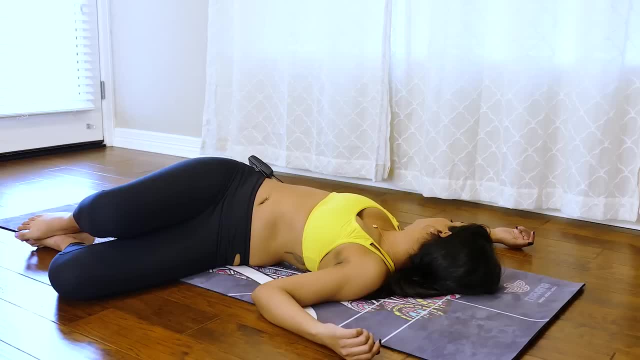 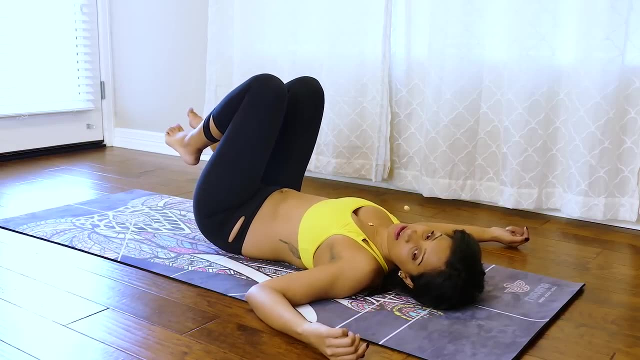 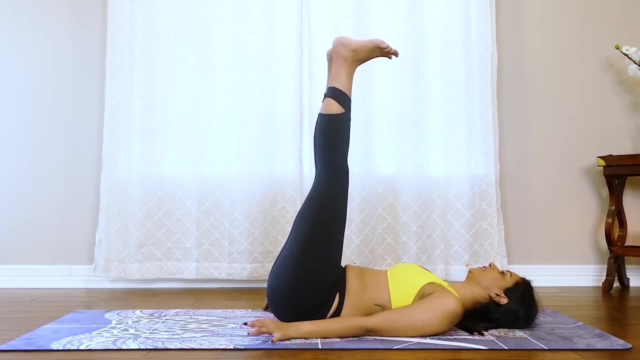 last breath and go ahead and on the next inhale bring those knees into the chest. we're going to take one inversion before our final resting pose. so a couple options for you. at home we can just bring the legs to waterfall, so pointing the bottoms of the feet up to the ceiling, if you want to take it a little. 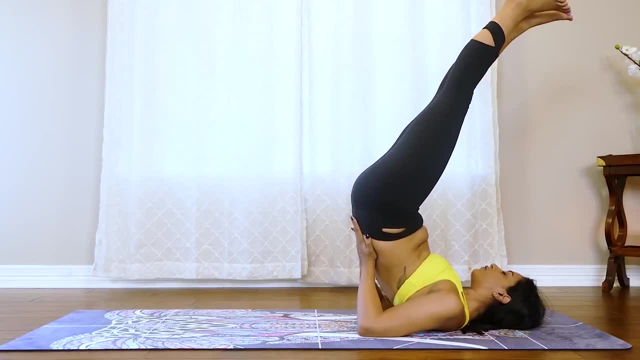 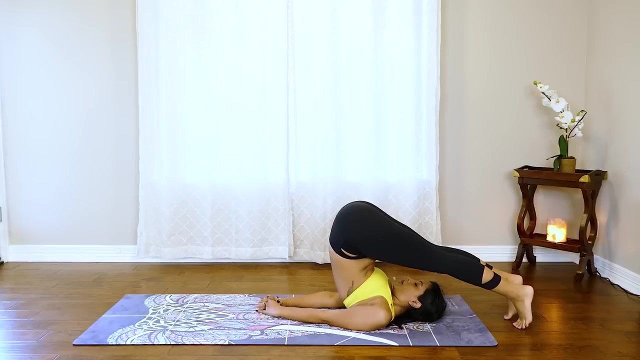 option to shoulder stand. so, coming up onto the forearms, make sure that neck is nice and long, using the arms to balance. if you want to take it all the way, go into your plow, pose legs over the head. three breaths wherever you are. last breath and from your inversion, slowly, slowly, again coming out the same way you came in, bring. 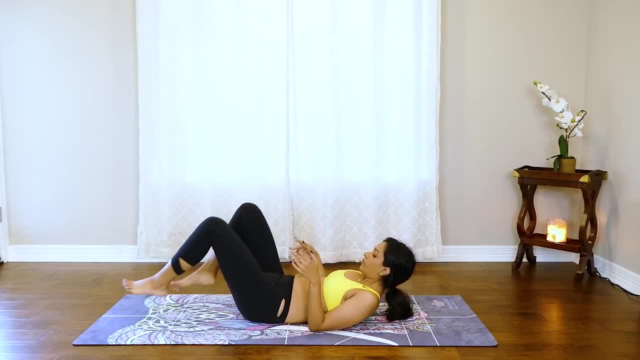 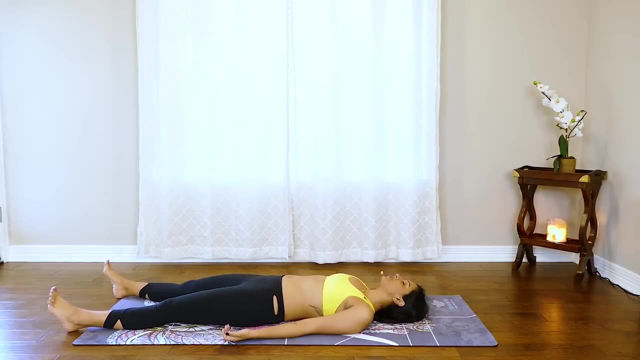 the feet to the ground, rolling the length of the spine. let the legs fall out long in front of you, arms come down by the sides, palms facing up- shavasana. let go of the breath here. just let them mat take the entire weight of your body for a quick flow like this. guys, you still want to. 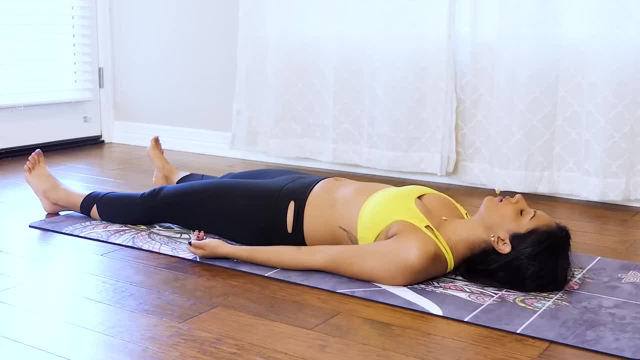 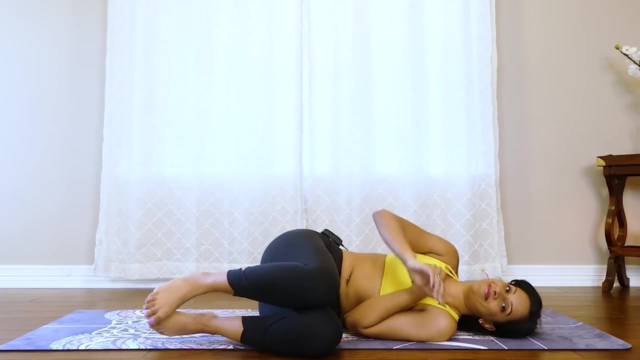 stay in your shavasana. you can stay here from anywhere from two to five minutes. when you're ready, you can join me, bring the knees into the chest, roll over to one side and we'll use our hand to push us up and down and we're going to take a deep breath in and we're going to